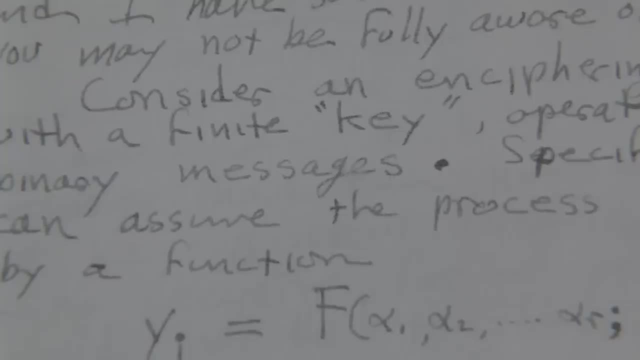 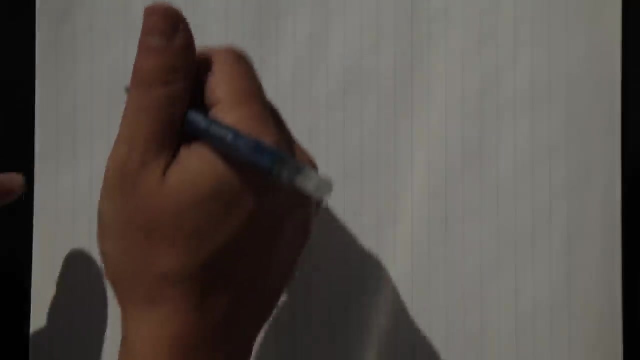 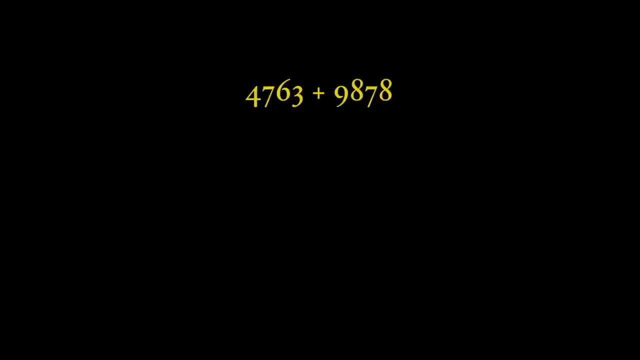 this concern in a letter to the NSA. In this case, he cared about code breaking First. he suggests that we look not at the absolute time needed to calculate any specific example, such as how long it would take to add two four-digit numbers, but instead look 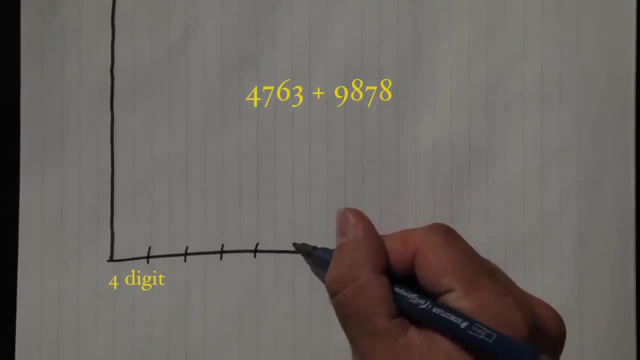 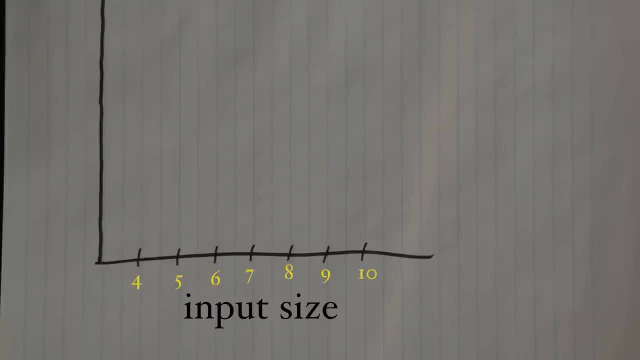 and so on. So we can look at how long it takes to add two four-digit versus five-digit versus seven-digit number. And instead of measuring this in terms of seconds, we should instead use the number of machine operations needed to generate an answer, or simply the number of steps. 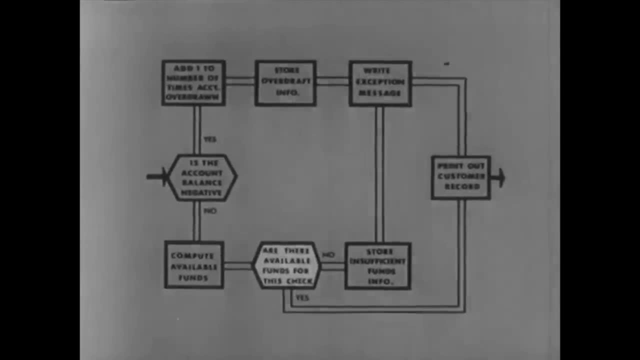 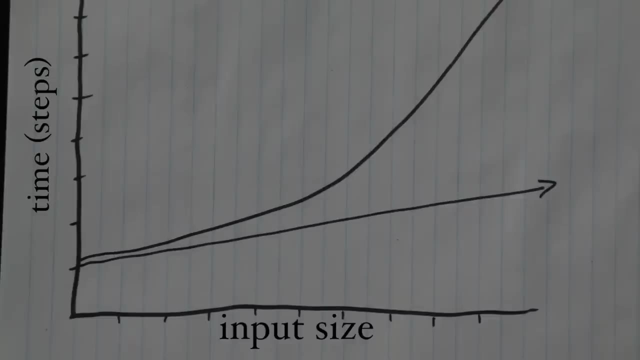 Another way to think about the number of steps is simply the number of state transitions the machine goes through, And then we can graph the growth of any operation sequence this way and get a curve representing how many steps any machine will demand. The question size or input size grows. 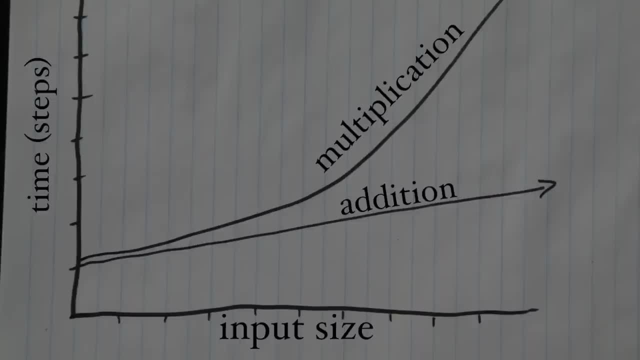 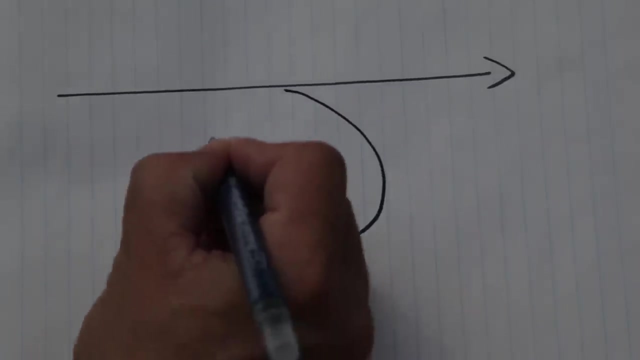 For example, addition grows more slowly than multiplication, which we can all relate to, because there is more rough work involved to get a solution, And so it was the shape of this growth curve that became a meaningful way to classify a problem. Now, one key reason this growth increases more sharply for some problems is the existence. 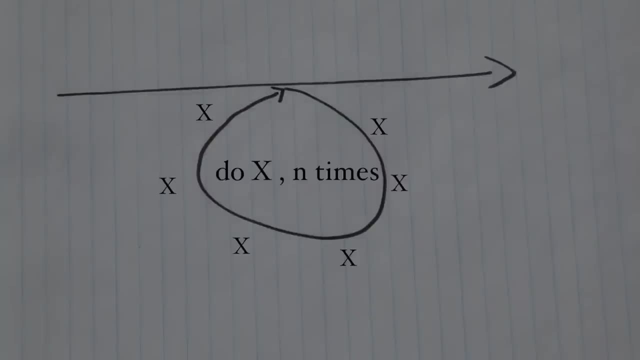 of loops in the algorithm being run by the machine. So often the number of steps increases. So the number of steps in a loop will depend at least on the size of the input. This leads to a straight line when we plot it on a graph: number of steps against input. 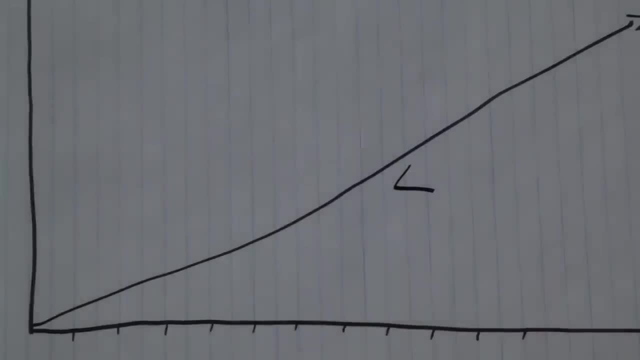 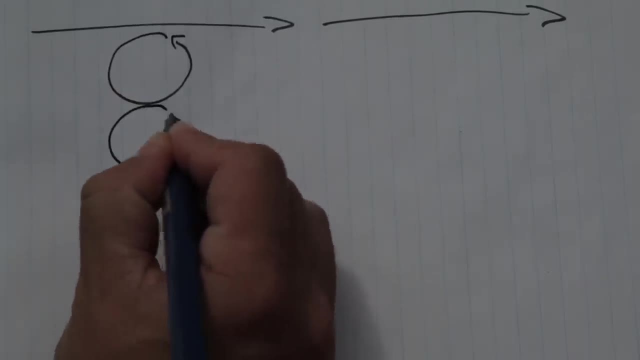 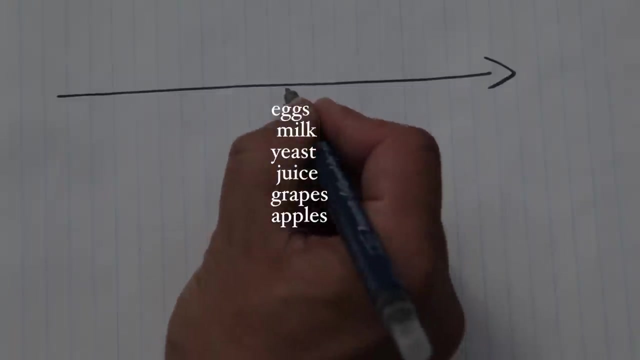 size, known as linear time growth. Yet more complex problems will call for algorithms that have loops within loops, known as nested loops. For example, we perform a nested loop when checking if a grocery list is complete For the first loop. we go through each of the first two loops. 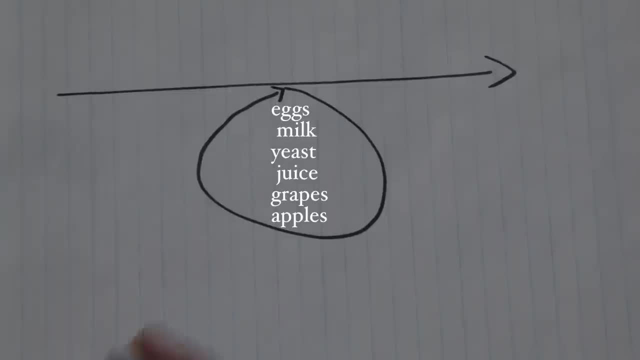 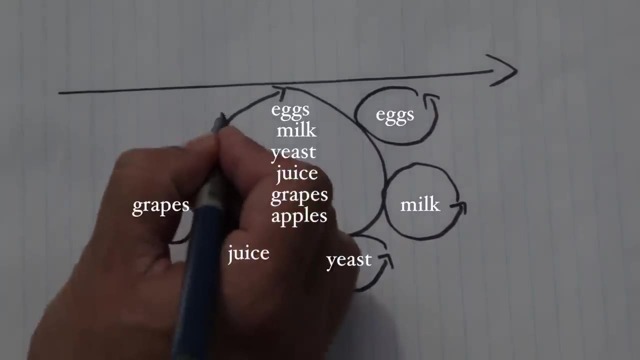 The difference between the first loop and the next loop is that each of the loops which we just looked at are nested loops, item on our handwritten list and then for each item in that first loop we perform a second loop, which is we scan our entire cart until we find that item. So if a grocery list is n items long, 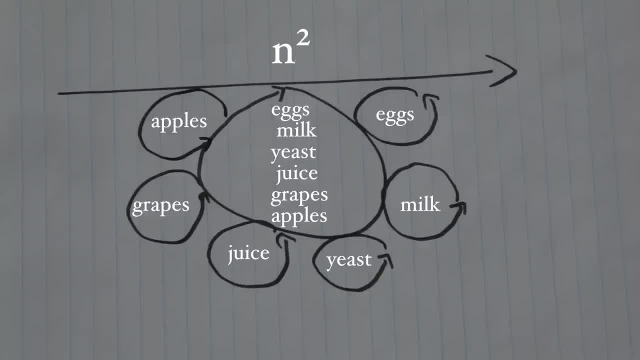 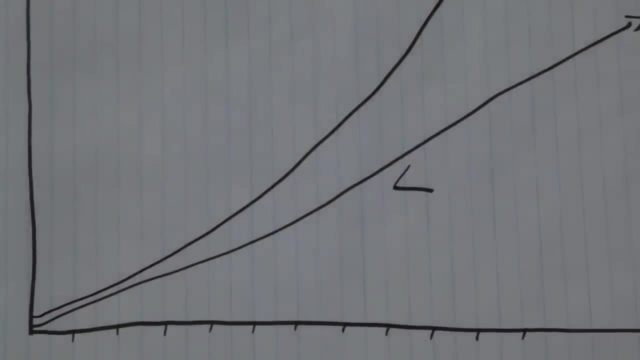 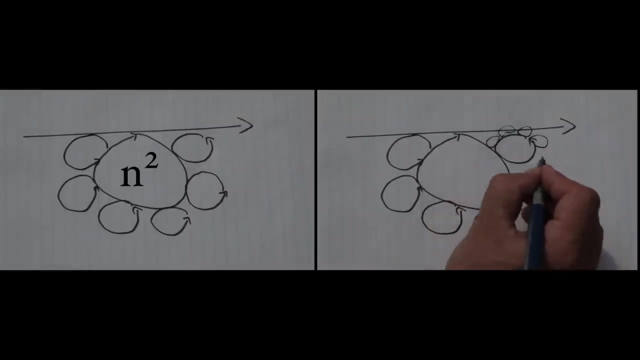 it could require n times n or n squared steps. Now, if we graph this structure in the same way, we instead get a curved line, and in our example it could be expressed by the equation n squared. and if the loop is nested more than two times, this exponent grows with each new depth. For 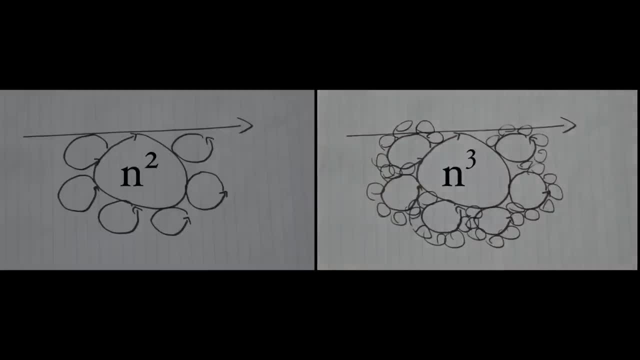 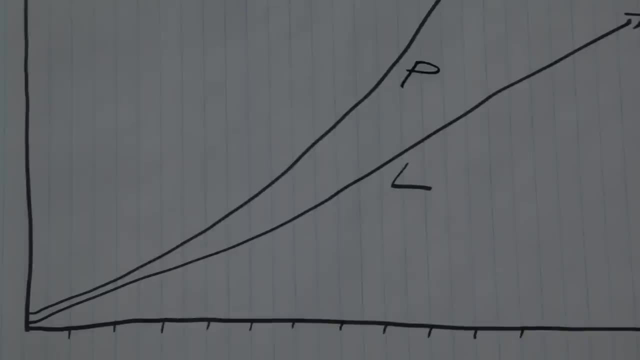 three nested loops, we'd get a growth curve n to the power of three, and so it was suggested that we call these kind of problems polynomial time, because the curves which represent their growth can be described using one or more terms of the form n to the power of k, where, in our example, n, 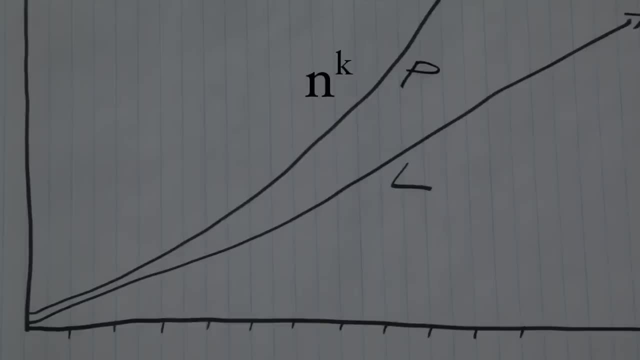 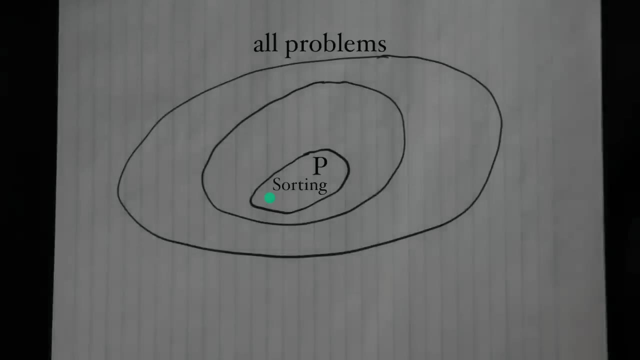 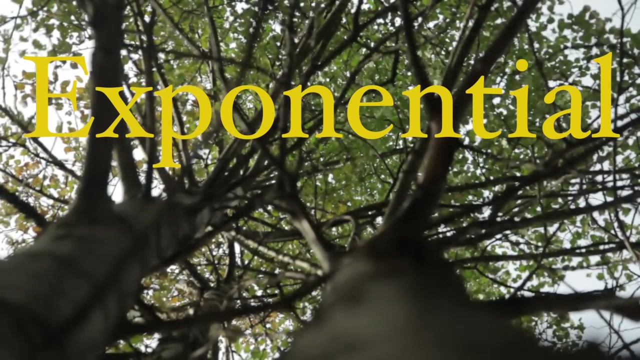 is the input length and k is the depth of the loop nested. And it turns out most problems we ask a computer to solve require polynomial time, for example sorting a list of numbers. but there was another kind of growth which caused us the real problems. For example, if we are trying to 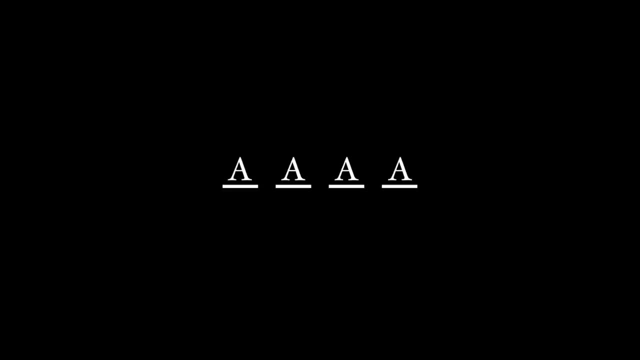 crack a password by blindly guessing all passwords and trying each one, then for each letter we have to try all other possible letters. This means the number of times we nest our loops grows with input size. So if we have, if the password is four letters long. 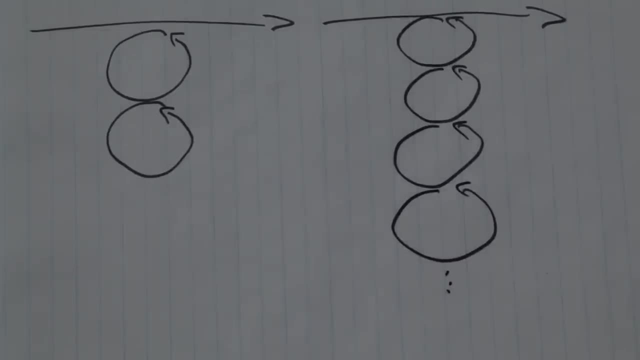 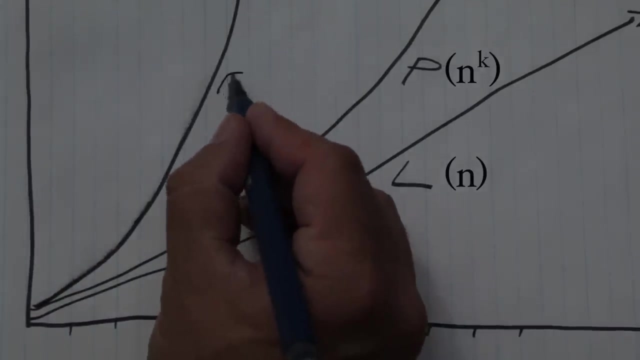 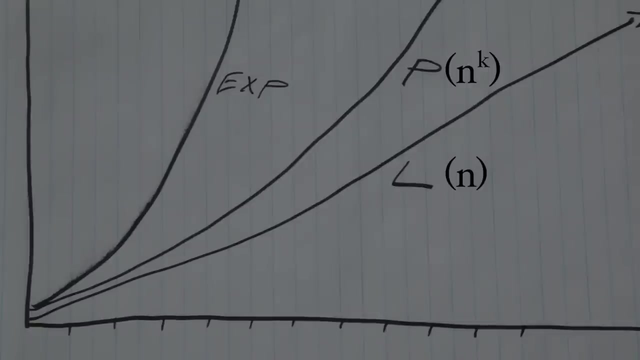 this requires four nested loops. Now, if we plot this kind of growth in the same way, you can see that the curve turns up more sharply than polynomial time. And we call this category of growth exponential time, because the curves which represent the growth can be described using one or more terms. 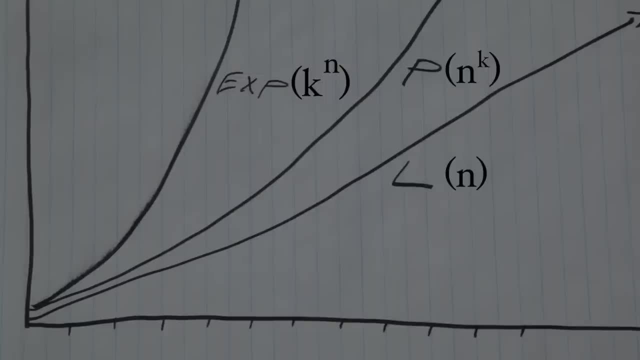 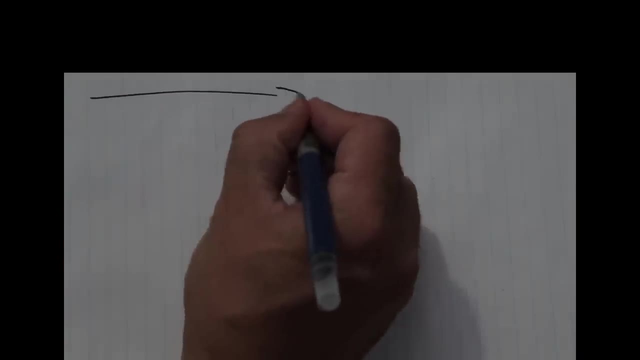 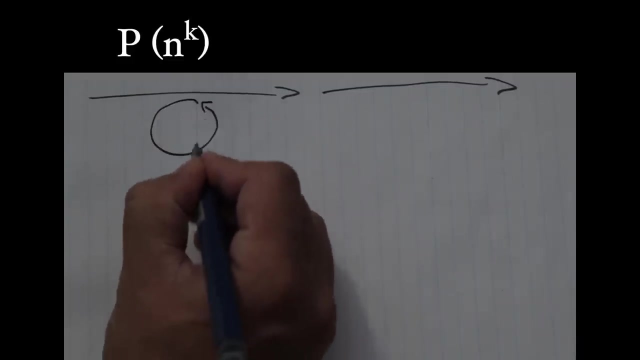 of the form k to the power of n. The key difference here is that in this case, the exponent grows with input size, And this is an important difference. so let's summarize using our example with loops With polynomial time algorithms: the number of loops in the algorithm. 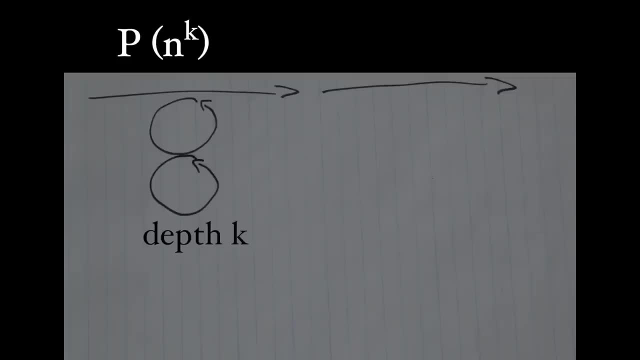 doesn't change when the input size grows. And increasing the input or n simply adds to the number of steps within each loop. But with exponential time algorithms the number of loops in our algorithm increases when input grows. Practically speaking, it doesn't take a large input. 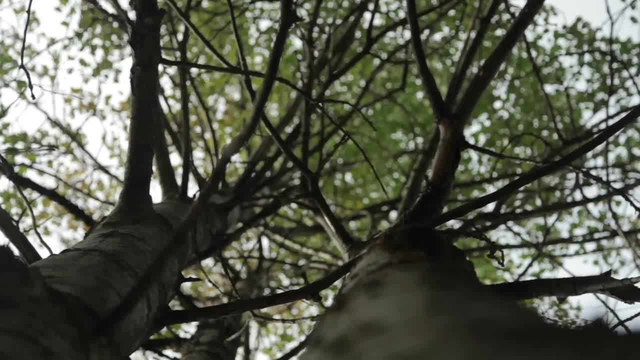 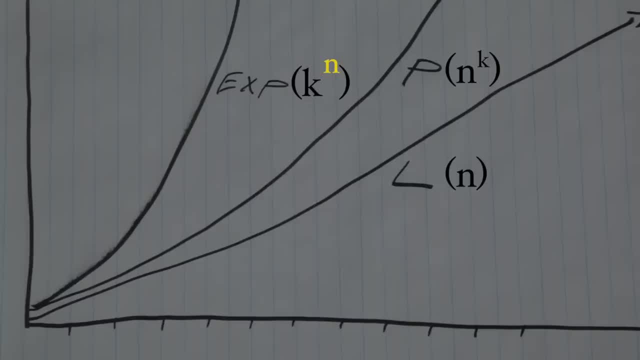 in the exponential case, to reach a point where the number of operations or loops exceeds anything a computer could handle in a practical amount of time. This difference between polynomial time problems, which we can think of as practical to solve in most cases, and exponential ones, which are never practical to solve, 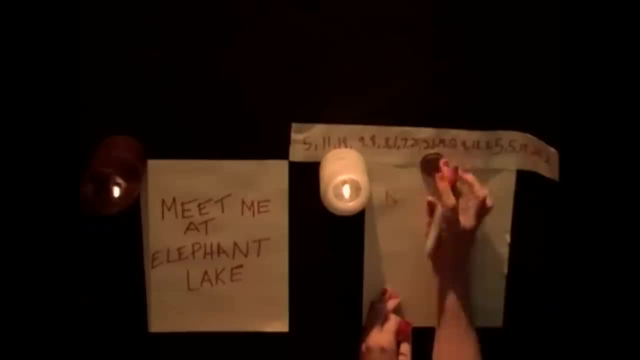 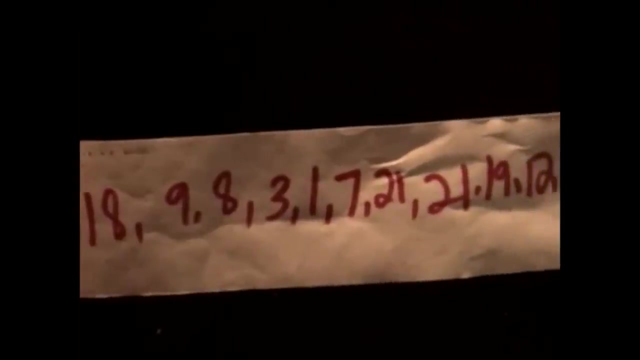 with large input is what interested Nash, Because he knew the process of encryption, which is scrambling a message using a secret key, was really fast to perform, While the process of decryption- unscrambling the message without knowing the secret key- 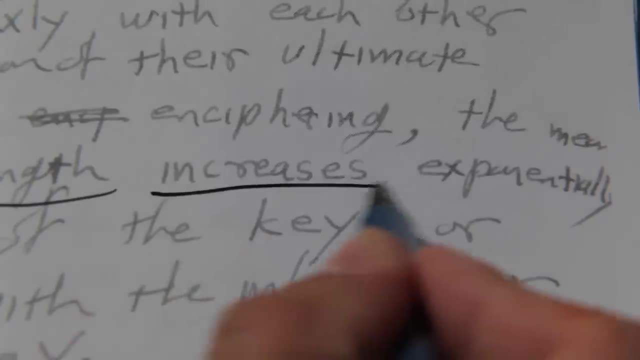 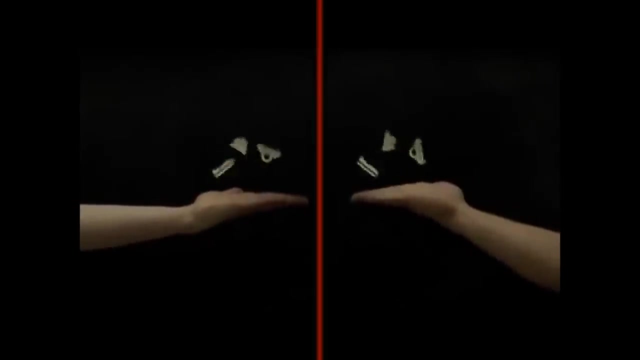 was slow or exponential time, since you'd have to resort to a long sequence of guessing to find that key. So he suggested to the government that as long as you kept your encryption key secret, you would end up with an encryption system. that was in his words. 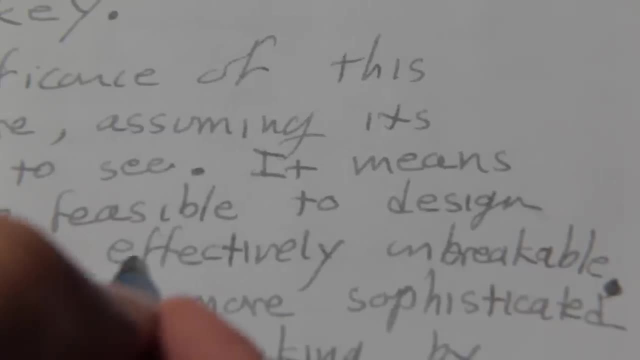 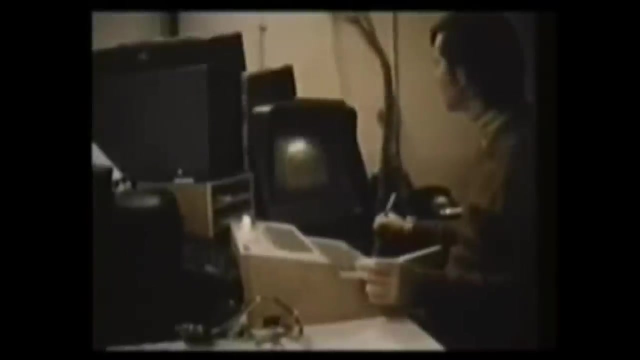 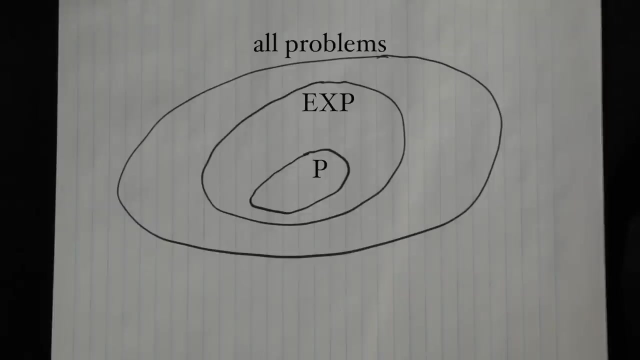 impractical for the enemy to break if we simply choose n to be larger, And no matter what domain computers are applied to, the interesting or important problems we want our computers to solve often require exponential time to solve using our best algorithms. But of course people worked hard to find algorithms. 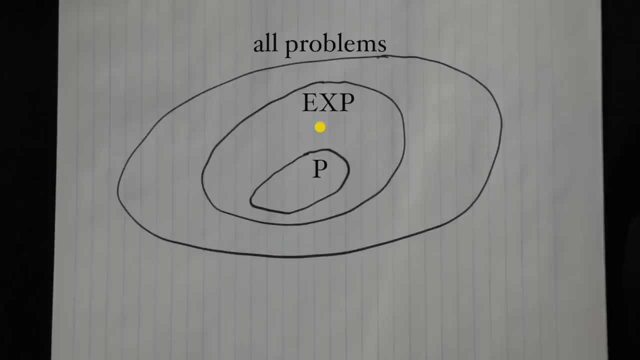 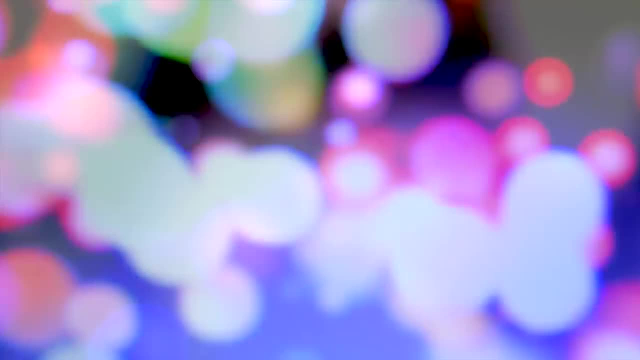 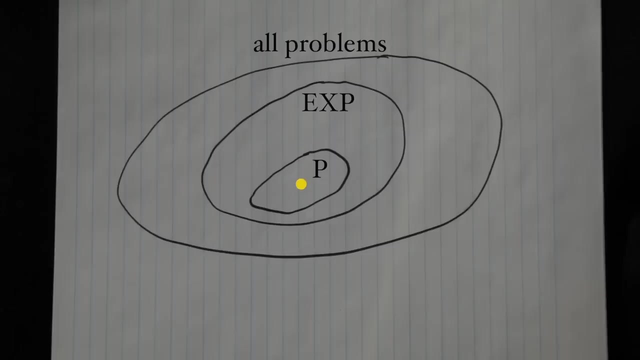 which could solve problems we thought were exponential time in polynomial time instead. And they do this by finding a clever shortcut to the solution, And when this happens, we say they reduced the complexity of the problem From the exponential category to the polynomial category. 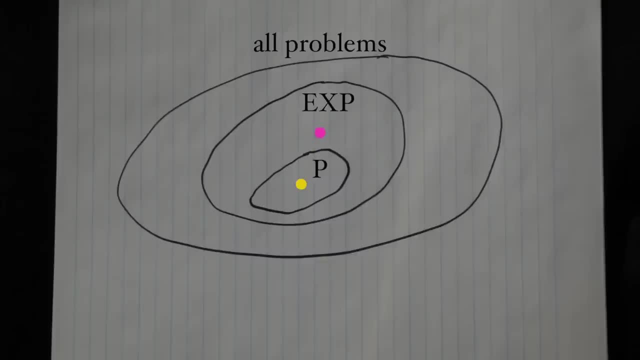 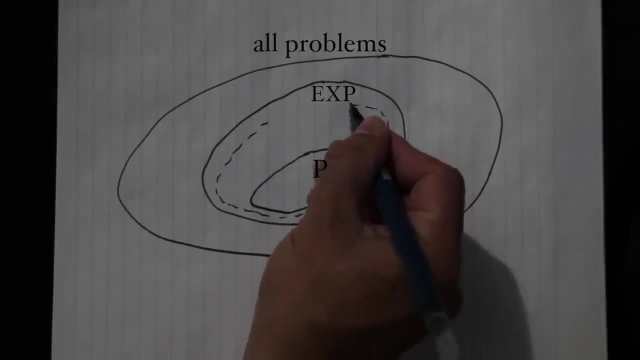 Yet many problems seemed irreducible, For example, finding the prime factorization of a number. What happened next is interesting, because people began noticing a set of these exponential time problems that seemed to have a special connection. They all share a quality we recognize in riddles. 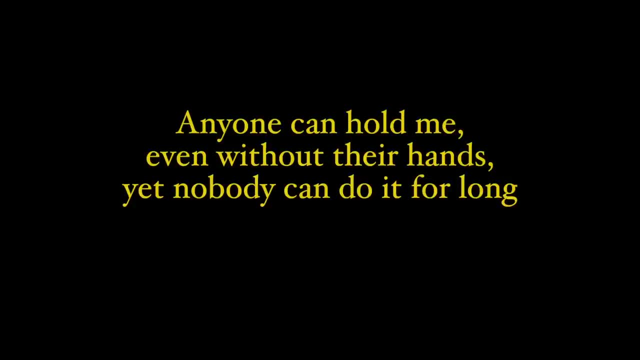 That is, they're problems which are difficult to solve but once a solution is given, they seem obvious in retrospect. Technically speaking, we say it's easy to verify if a riddle is correct. And these hard to solve but easy to verify problems. 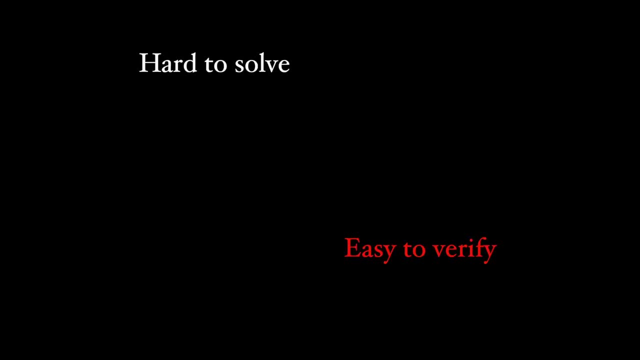 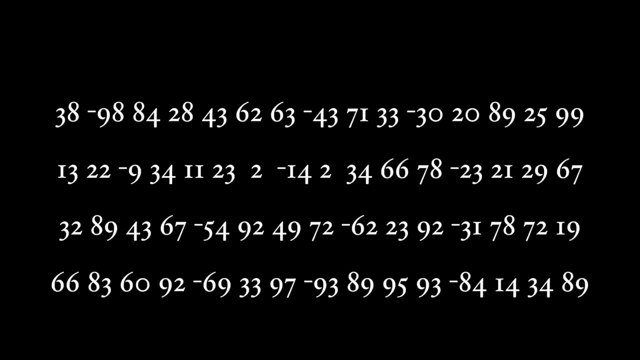 were popping up everywhere in the world of computing in the form of decision problems. For example, given a collection of numbers, can you identify a set of them that adds up to zero? Solving this problem is hard. Yet if you are given a solution to this problem, 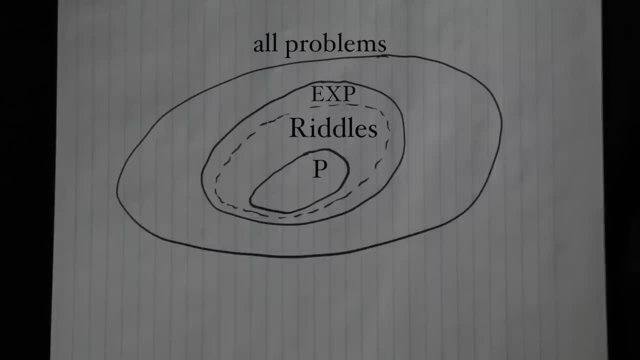 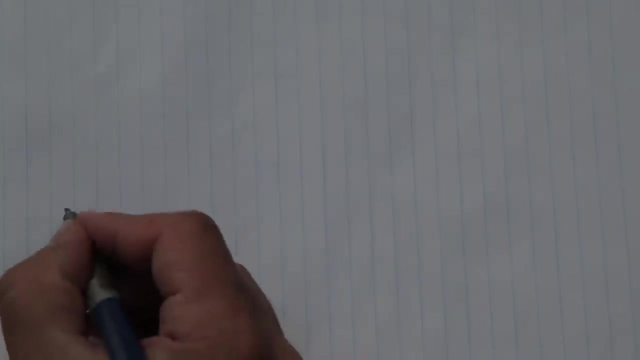 you can certainly verify it's correct very easily. And they gave this category of problems a really strange name: NP. And here's why People considered how these kinds of problems could be solved in polynomial time in theory, Because in theory you could just. 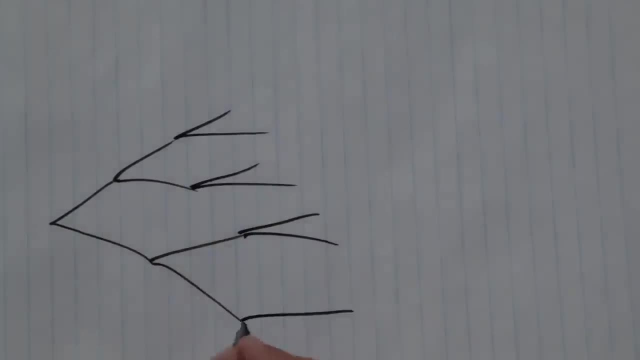 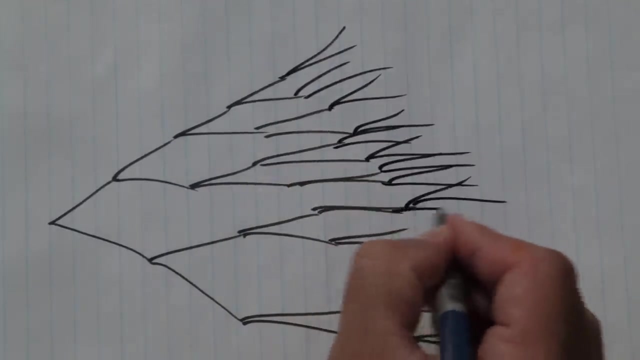 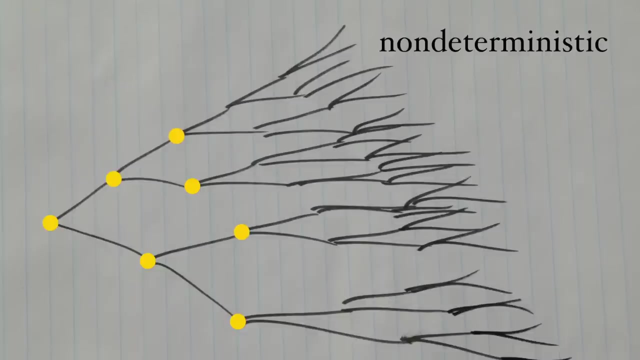 use the fast verification procedure in parallel on all possibilities and just check if there is a correct one. Think of it as guessing In parallel. And this would only be possible on a theoretical machine which is able to make multiple decisions at the same time. 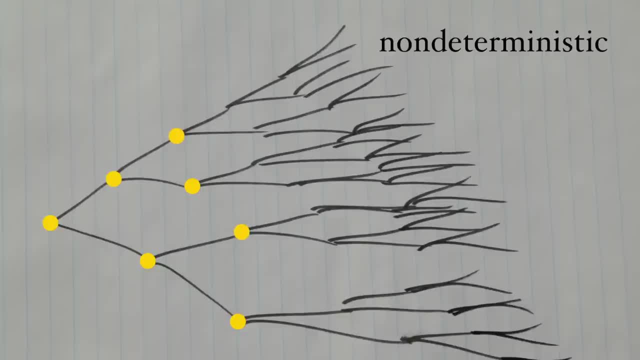 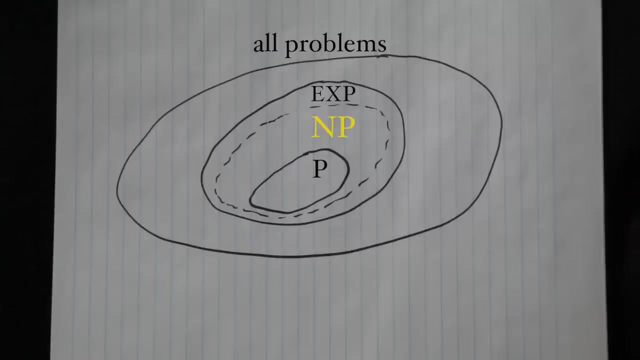 We call this theoretical machine a non-deterministic machine, compared to our actual machines, which we call deterministic because they can just jump from one state to another in a linear sequence. And this is why we call this set of problems NP. It stands for problems which are solvable in polynomial time. 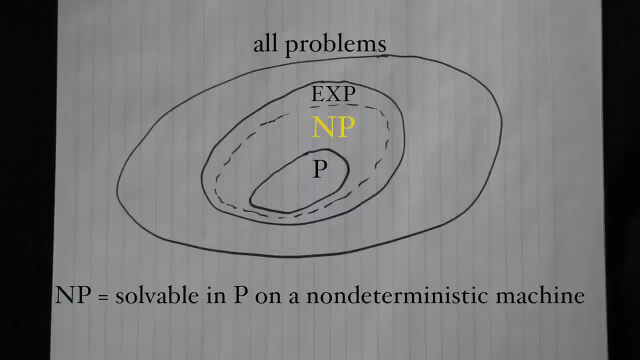 using a non-deterministic machine, Or simply non-deterministic polynomial time. It contains hundreds of important problems we face every day in computing, But since this non-deterministic machine doesn't exist, it is thought that the problems in NP. 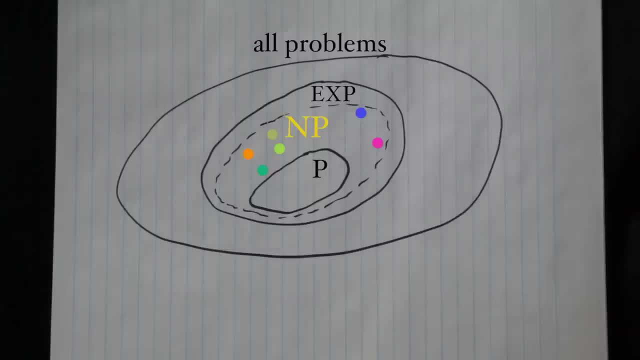 will always be exponential time to solve with our regular deterministic machines. That is, P does not equal NP. But there is one last twist to this story. People have noticed that many problems in this set NP can be reduced to a set of problems that can only be solved in polynomial time. 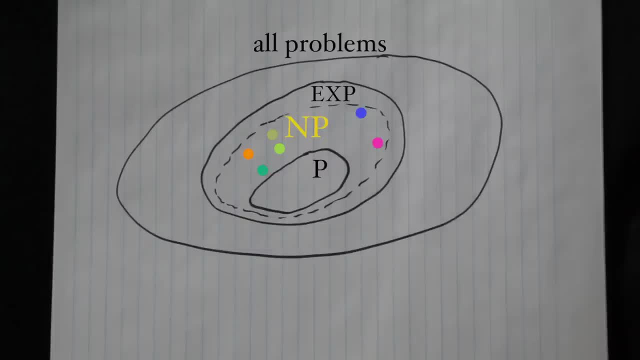 And this is why we call this set of problems non-deterministic machines. NP can be reduced to each other, And that's because they share some structural similarities, And so this set of interconnected problems is growing problems we call NP-complete. So solving any one of these NP-complete problems, 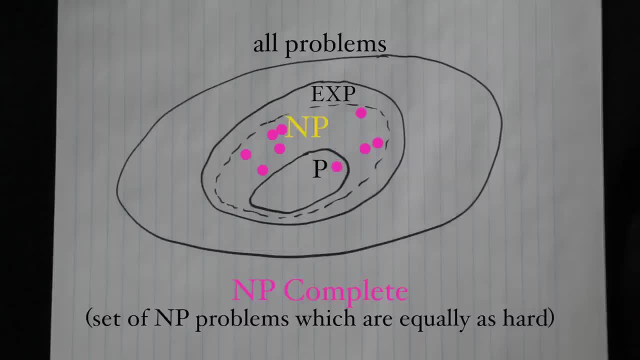 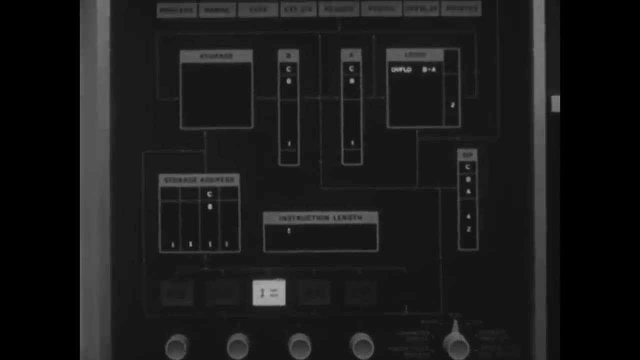 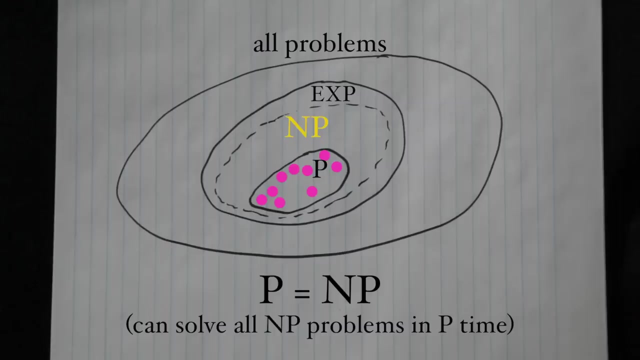 with a fast or polynomial algorithm would mean you also had a fast algorithm for every other problem in NP. A huge percent of the work that computers are doing today would simply vanish. Though most believe it's not going to happen, The other approach is to prove that this set of NP-complete 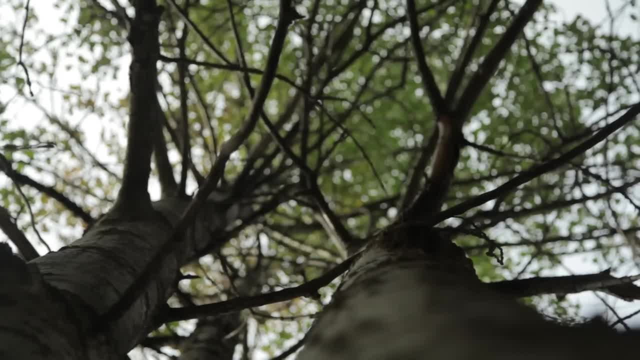 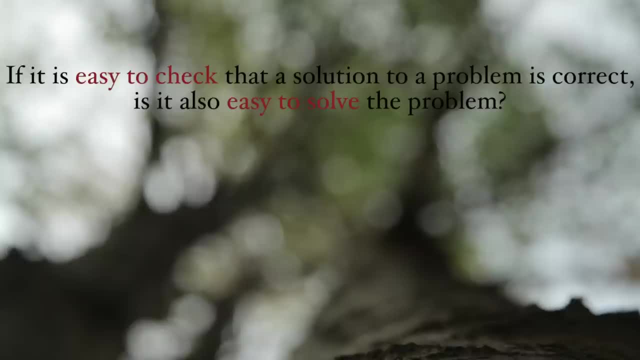 problems will remain hard and will be forever out of reach, And there is still a million dollar prize for anyone who can come up with a solution to this. It remains the most popular question in computer science today, And it all comes back to the initial dream.